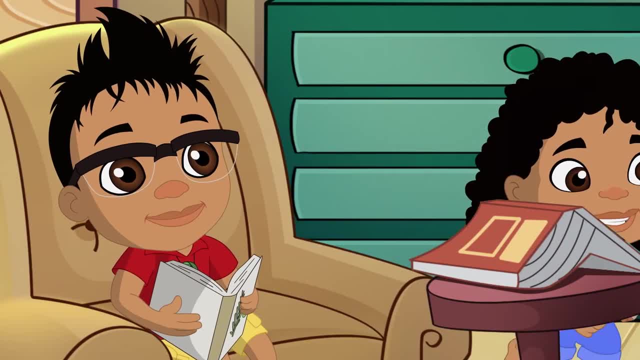 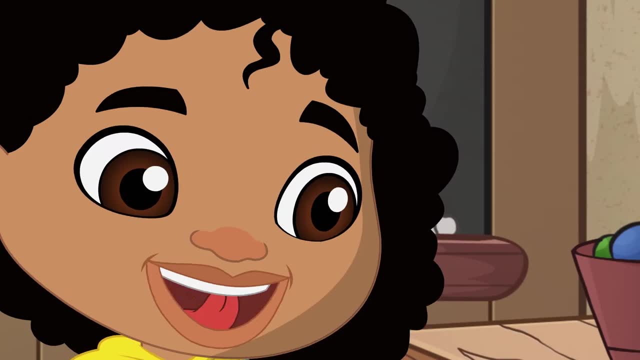 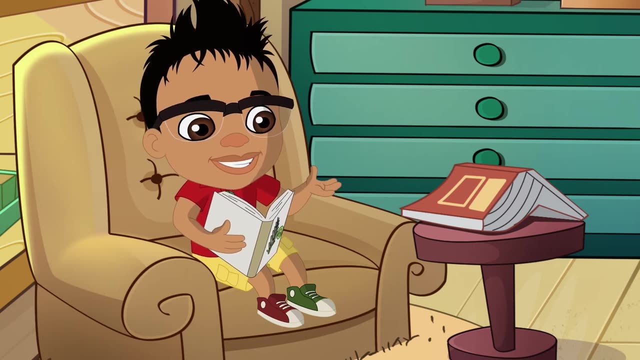 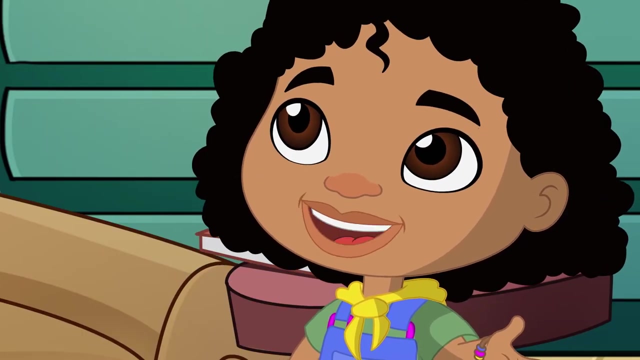 Have you ever noticed, when you hit different objects, they make different sounds? Yes, I was just observing that, Newts- Or should I say hearing. that Isn't it great. Why do different objects make different sounds? Well, that's because it depends on what the object's made of. 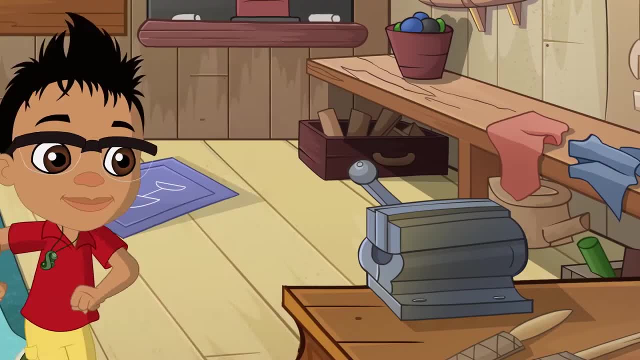 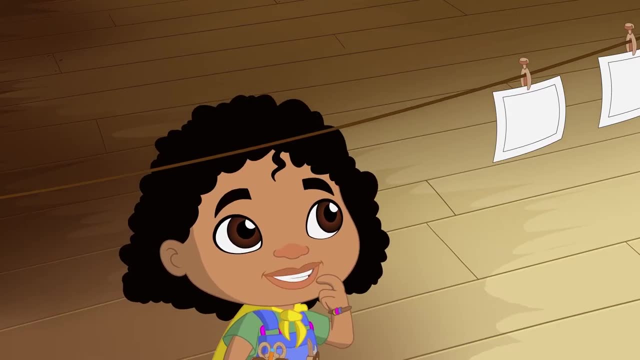 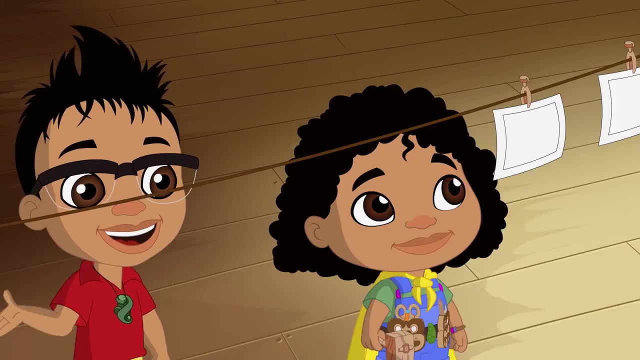 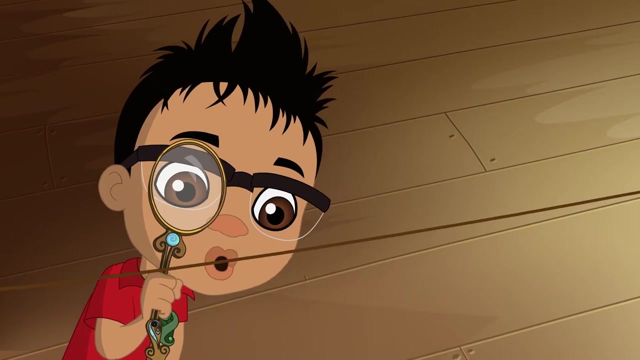 Hard, soft, solid or hollow. Wow, that was an interesting sound. That was an interesting sound. Do it again, please, Newts. The sound seems to come from the way the wire moves. I've got a great idea. 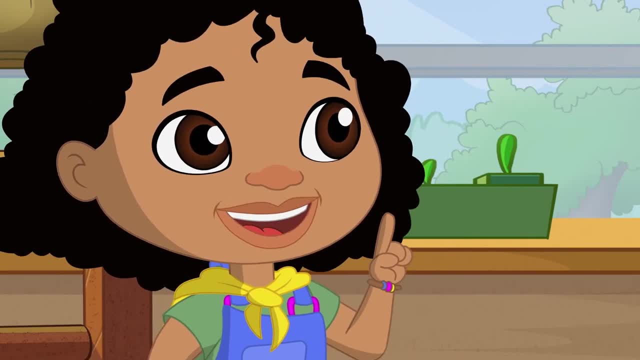 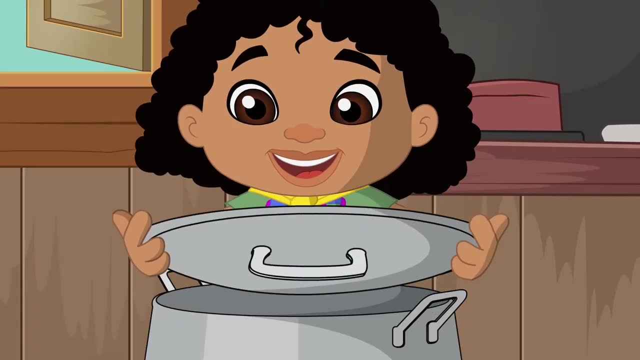 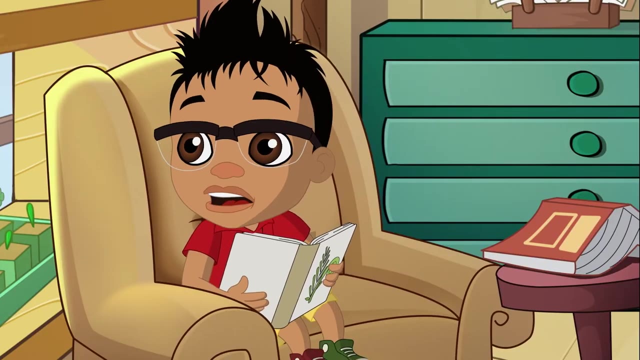 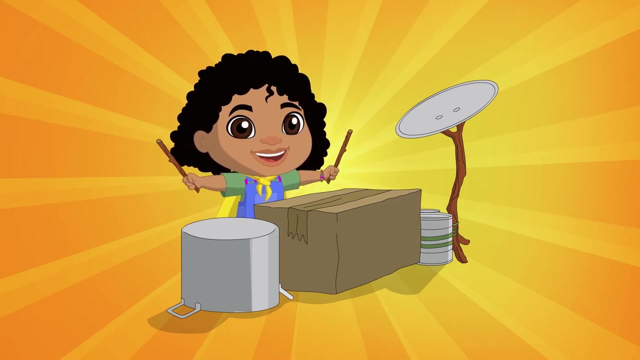 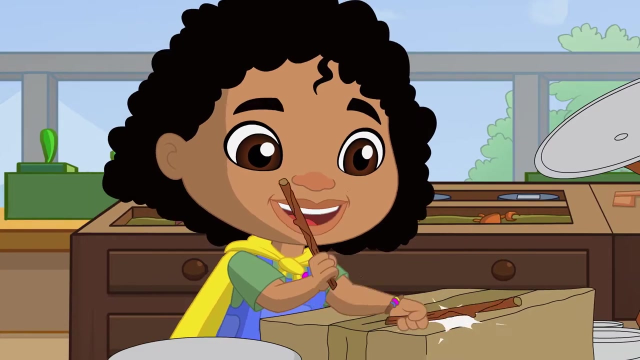 I'm going to get lots of different objects together and make something. I'm Anna, Yes Huh, Presenting my latest invention: Newts' noise-creating drumming machine. One, two, three, four, Do you like it? Darwin? 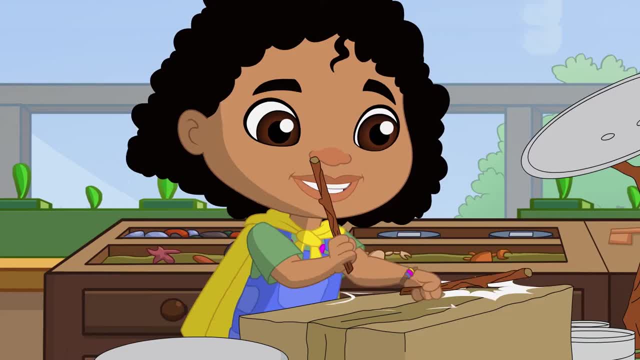 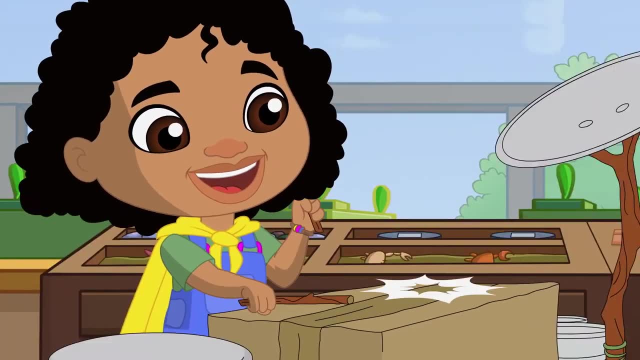 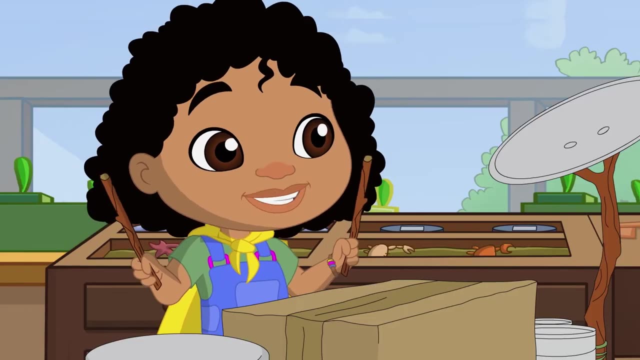 It's amazing. What did you say? It's amazing, But a bit loud. Sorry, I can't hear you. I said they're a bit loud, Darwin. I think you're being a bit loud. Sorry, Newts, But I'm trying. 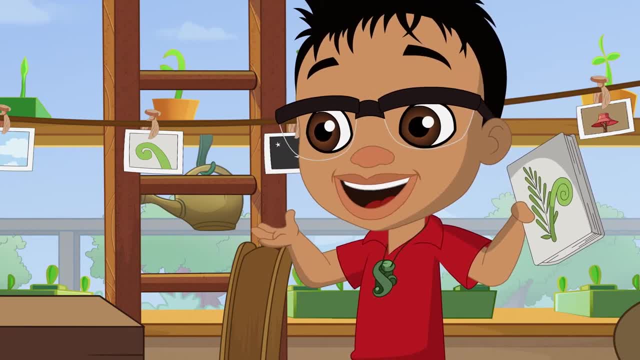 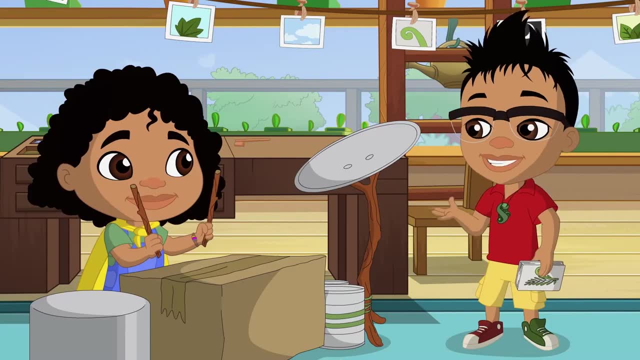 I'm trying to read this book and your drumming makes it hard for me to concentrate. Oh, I am so sorry, Darwin. It's okay, Newts, But how about I help you set up your drum kit down in the garden shed? 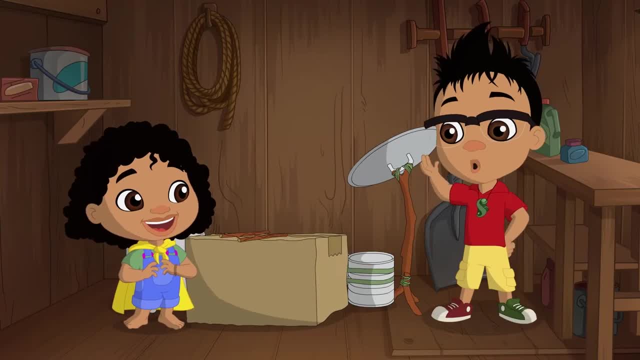 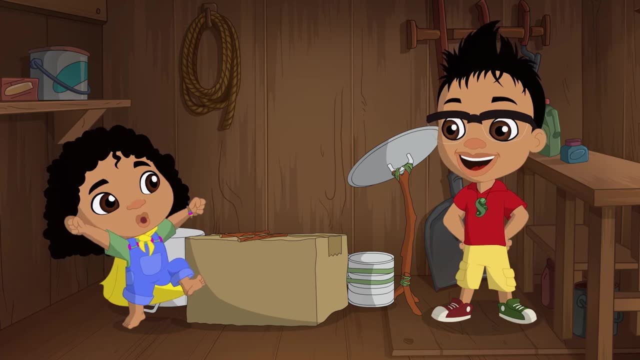 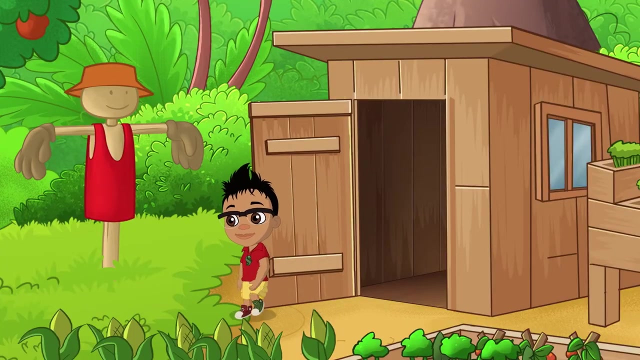 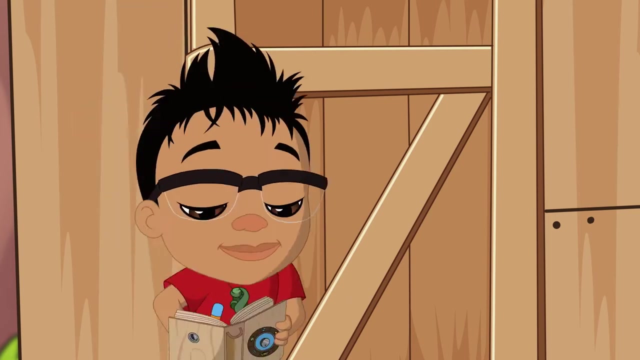 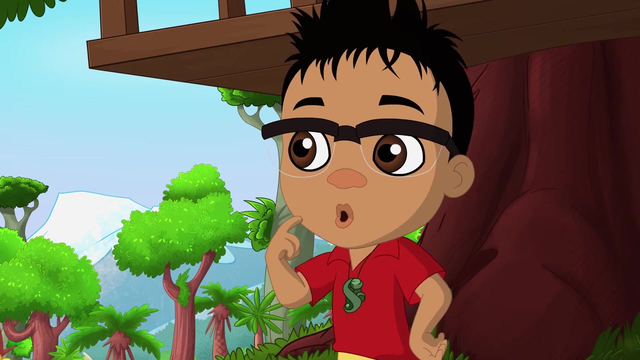 That's a great idea. Now you can make as much noise as you like, Newts. Thanks, Darwin. Wah-hoo, Ha-ha. And that was the last of your. And the further away I go, the quieter it gets. 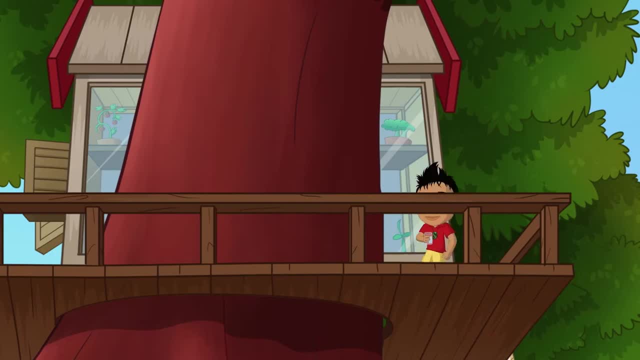 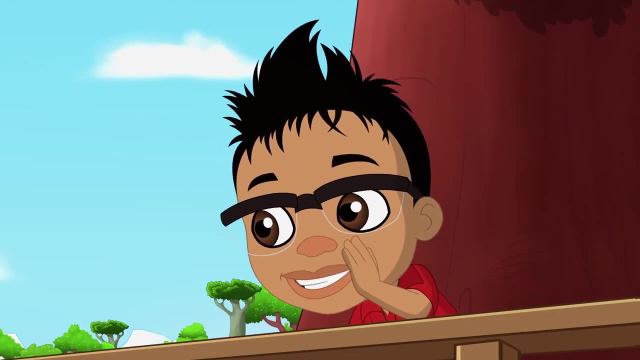 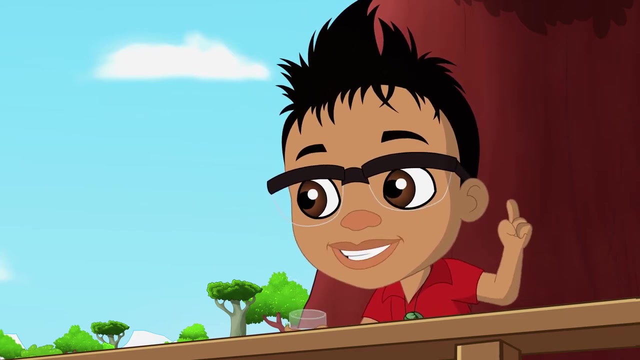 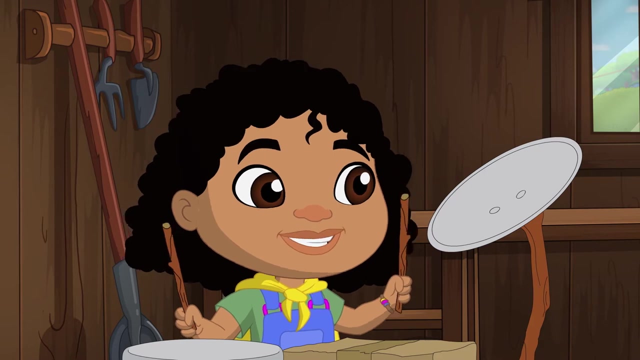 I wonder if Newts is thirsty too. Newts, Would you like some water? Newts, She can't hear me calling. For the same reason, I can't hear her drumming. Hey, Darwin, My drumming's not too loud, is it? 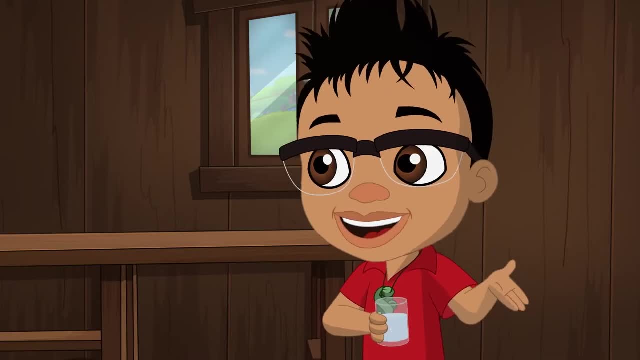 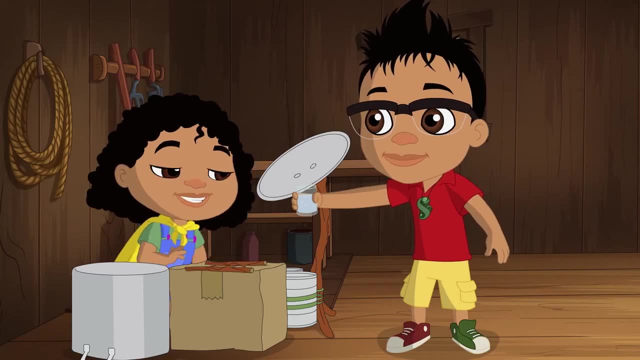 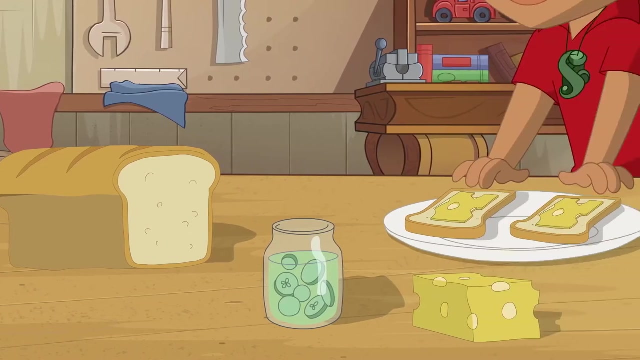 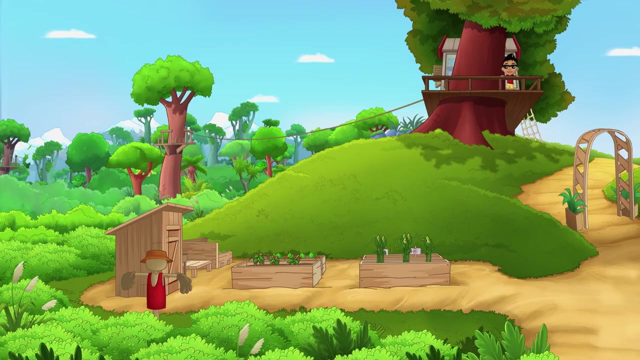 No, With the shed door closed and you being further away, it's not loud at all. Great, Would you like a glass of water? Thanks, I'm really thirsty. Newts, Do you want Pickle with your chase? She still can't hear me. 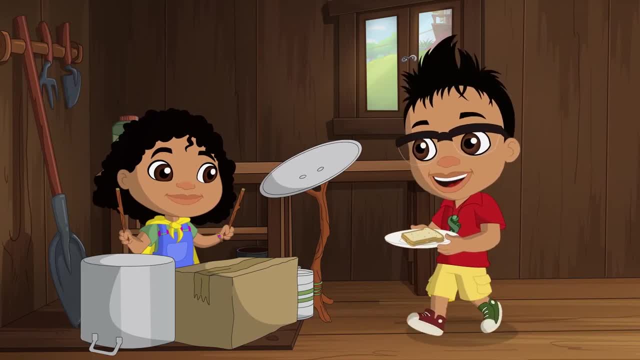 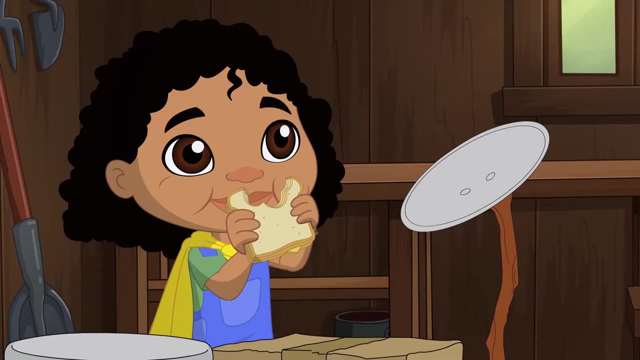 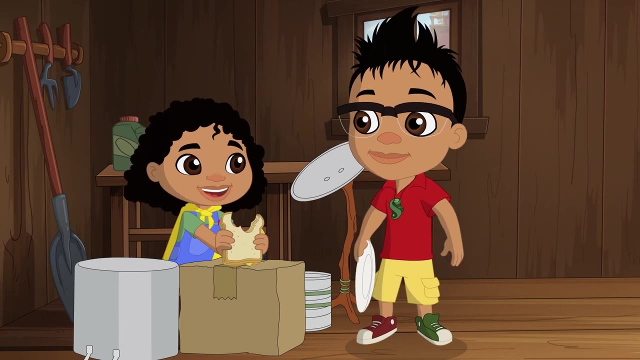 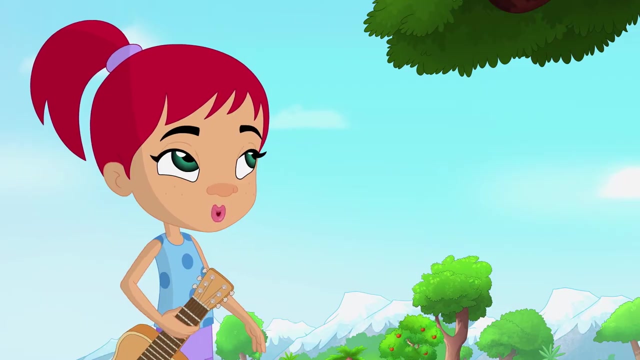 Your drumming's getting really good, Newts, Are you hungry, Really hungry? Thank you, Darwin. this is my favourite Cheese and Pickle, Or, as I like to call it, Chickle. Kia ora Darwin, Oh kia ora Henny. 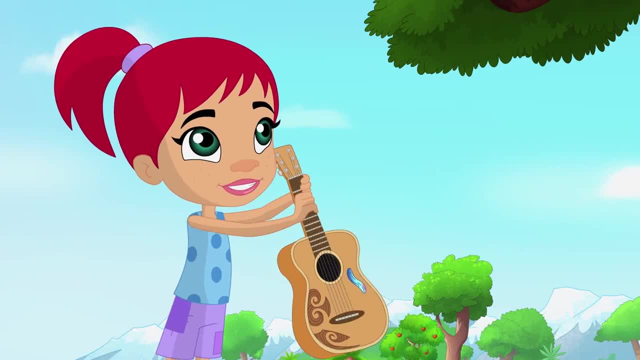 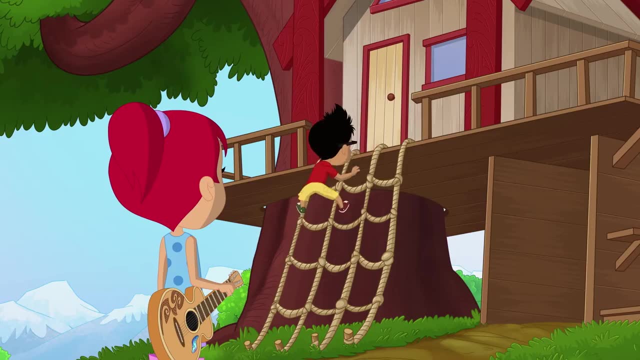 I heard some drumming, so I bought my guitar. However, for a sing-a-long, A lieta Newts will love that The drums are this way. We put the drums in the shed, so it's not so noisy in the treehouse. 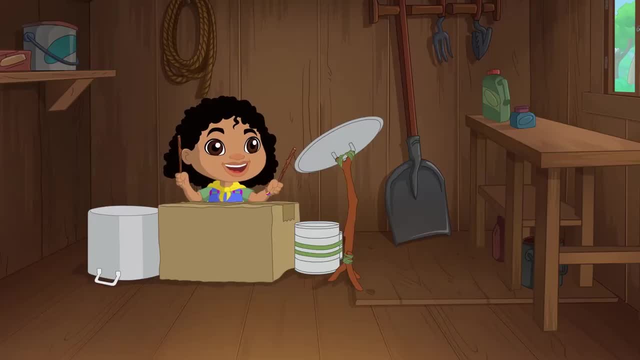 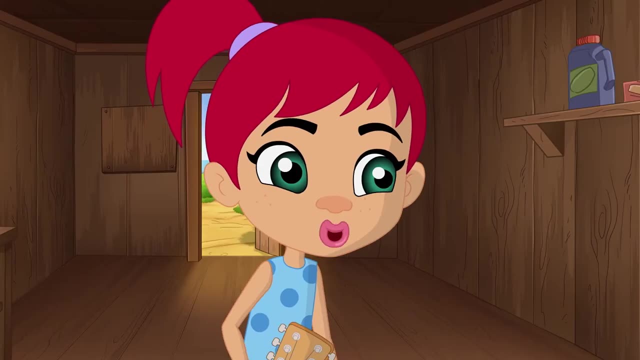 Clever idea. Yeah, Newts, you have a visitor. Oh kia ora, Henny, Do you like my drums? You're so clever, Newts, making your own drum kit. I brought my guitar, Huh. 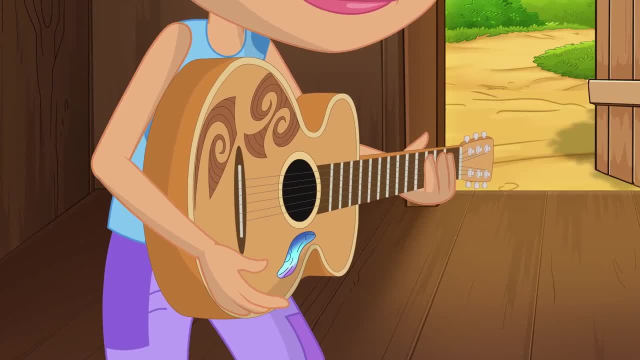 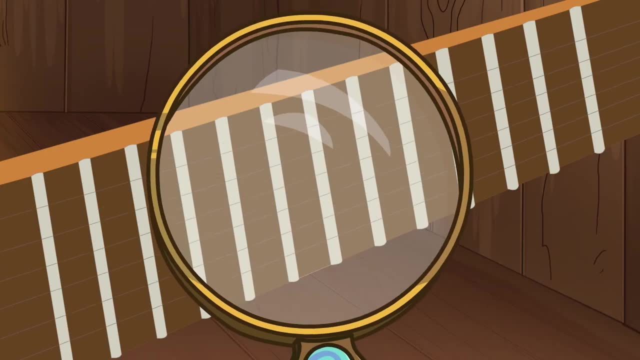 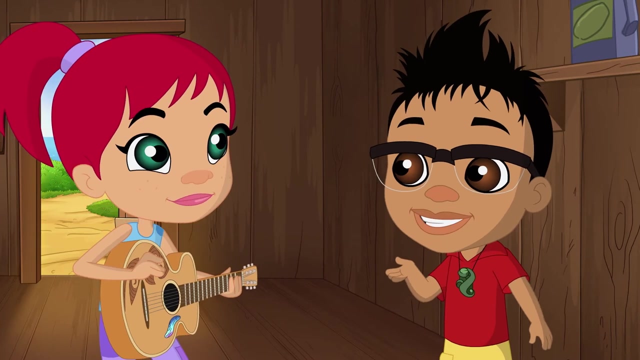 So we can play music together. That sounds beautiful. And look, Te Tiro, The sound is vibrating along the strings. What does vibrating mean? When something shakes quickly, like this guitar string, The sound vibrates the wire and travels along it. 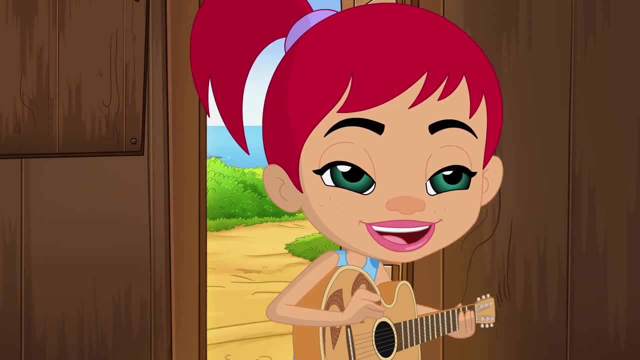 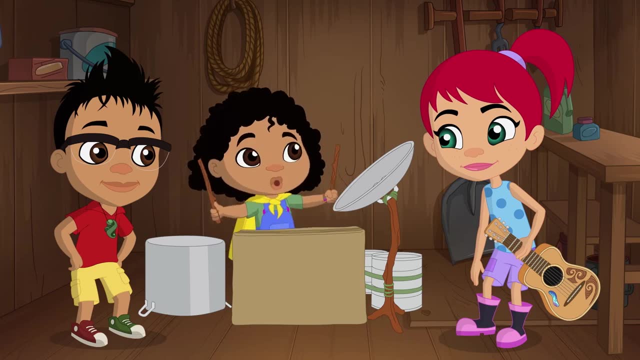 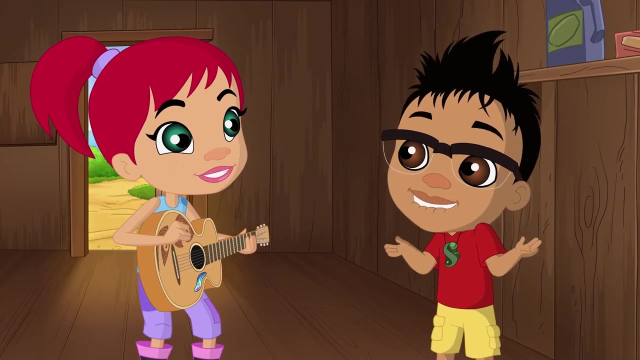 That's how we hear. The sound makes the ear vibrate, just like my fingers make the strings vibrate. Look, Te Tiro, I'm vibrating too. Mmmmm, Kind of Have fun, you two. I'm going to finish my book. 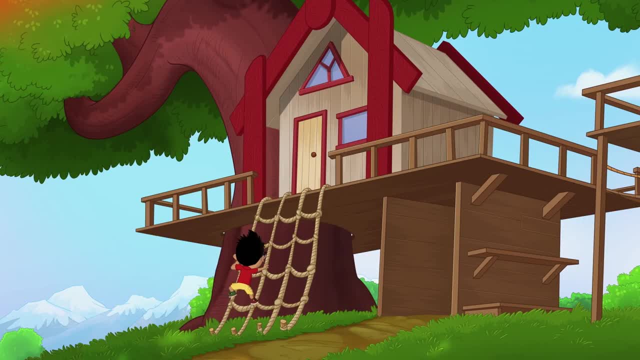 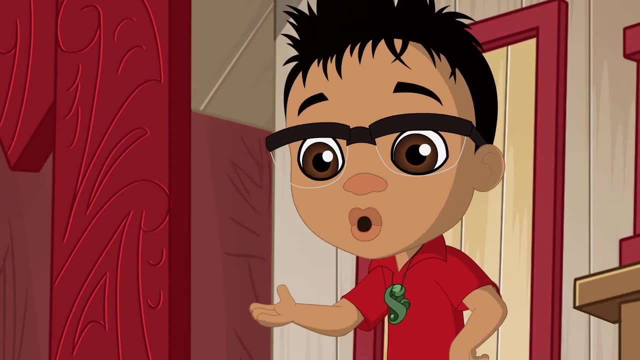 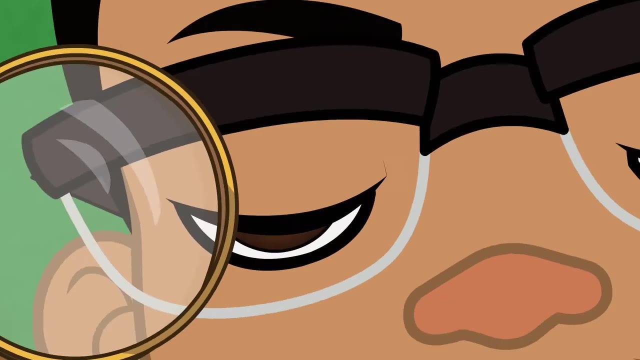 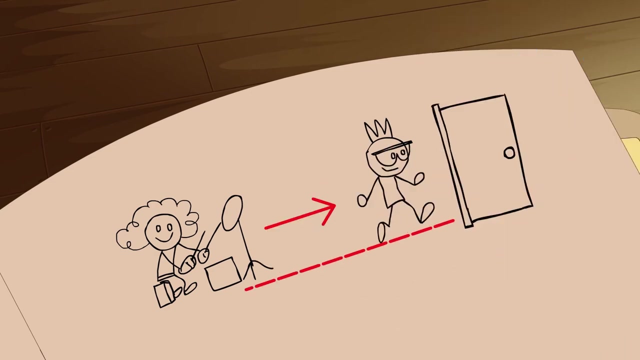 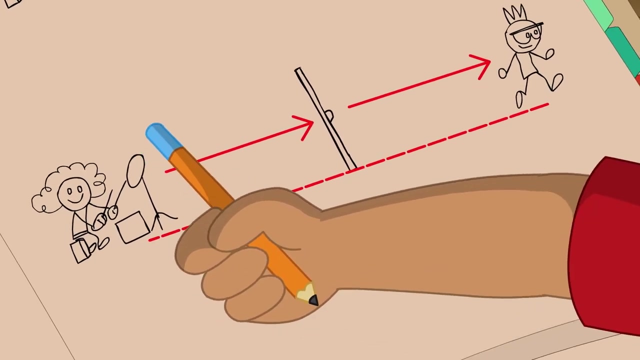 Call me when you're ready to perform. Going up and down to talk to Newts is hard work. There must be a better way. Let's science it. When sound travels through the air, it gets quieter as you move further away. And when you shut a door, it gets quieter too. 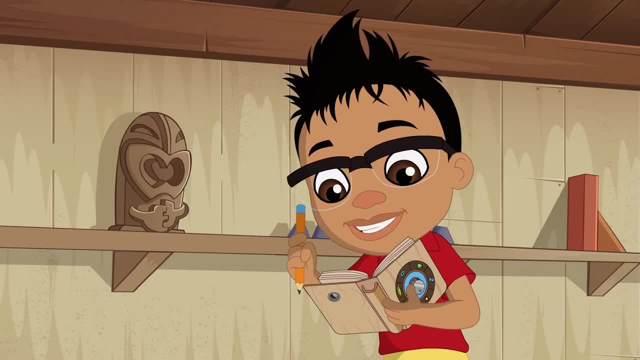 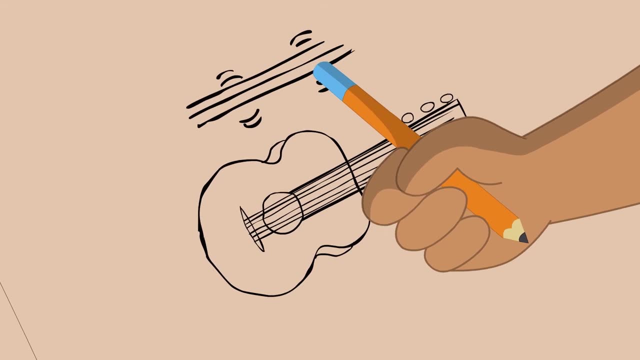 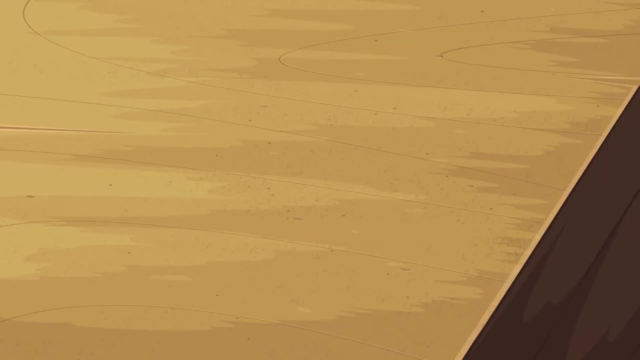 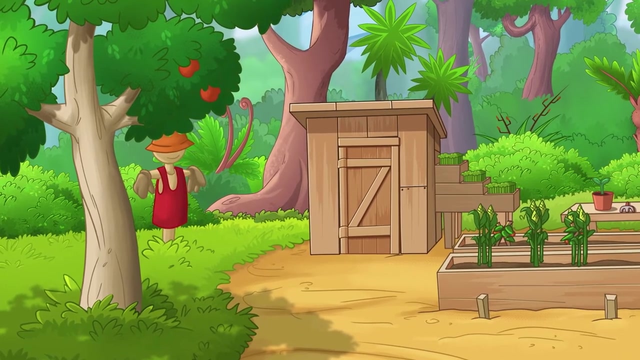 So I could hardly hear Newt's drumming and she could not hear me calling to her. But I also learned that sound can vibrate along a thin wire, like Henny's guitar, which gives me an idea: Perfect. Hey, Henny, we need to perform a song that Darwin will like. 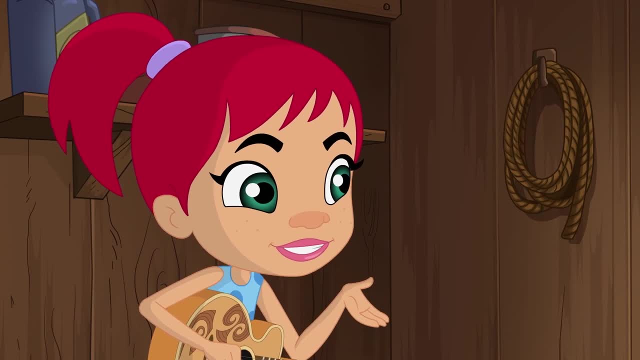 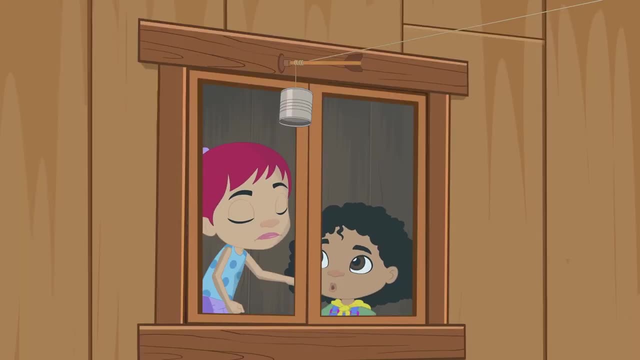 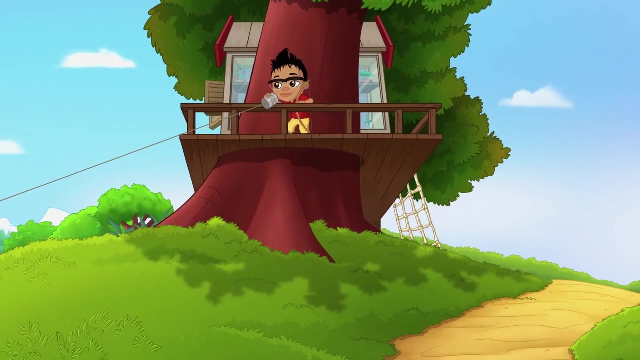 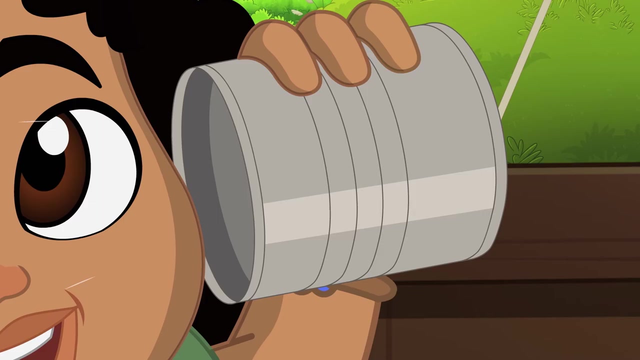 Hmm, I know, Why don't we write our own. Let's write our own song for Darwin. Pull the string tight, Hmm, Testing, testing, One, two, three. Can you hear me Over? I can hear you Over. 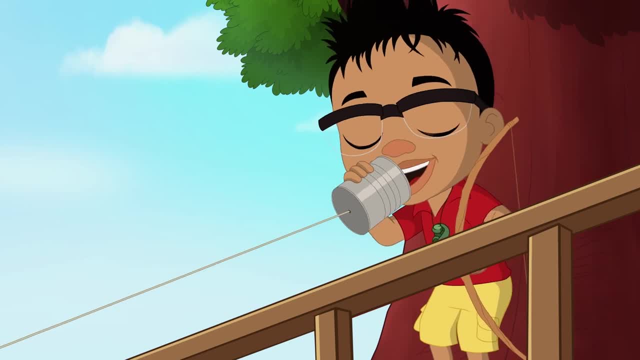 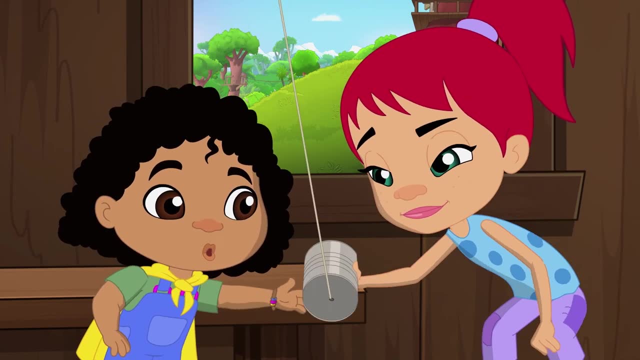 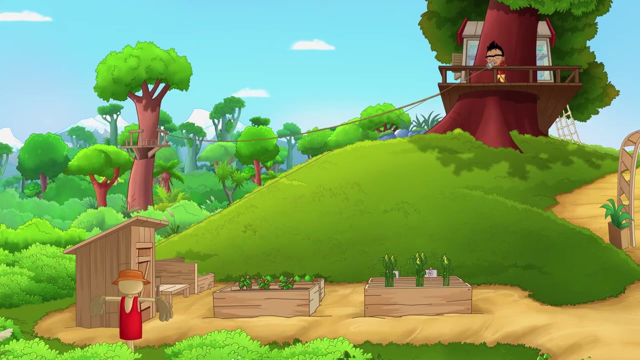 And it's amazing Over Presenting my Tin String Sound Conductor Device. Over What a great invention. Over How does it work. Over My voice vibrates along the string so you can hear me at the other end without me having to shout. 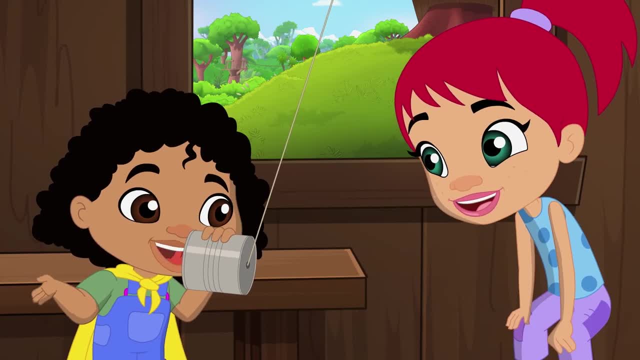 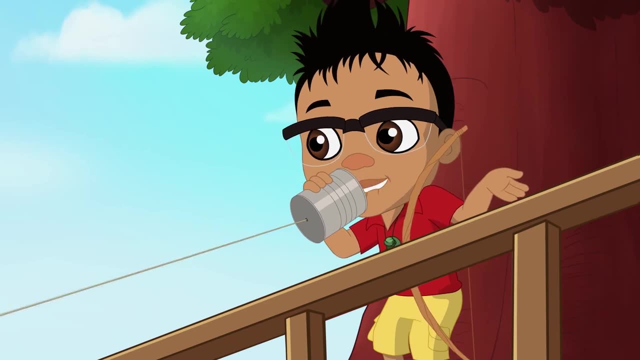 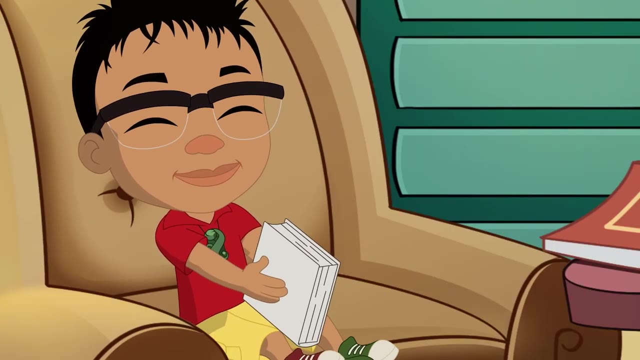 Over And the sound vibrates back along the string, so you can also hear me Over. Exactly, Call me when you're ready to perform Over. Turn out for now Over. Hmm, Hello Kia, ora. One, two, three, four. 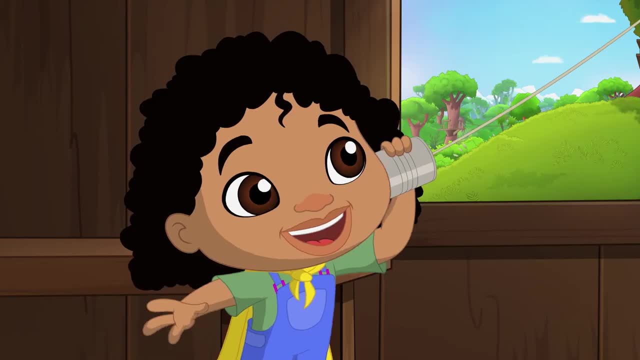 Testing. testing One, two, three. One, two, three. Can you hear us sing A B C. A B C. Do you hear the sound when I sing, When I sing Through the air and down the string? 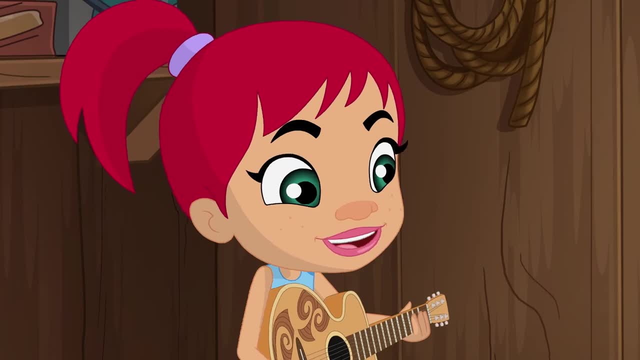 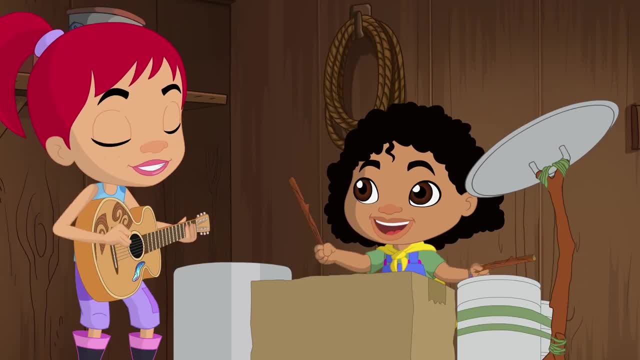 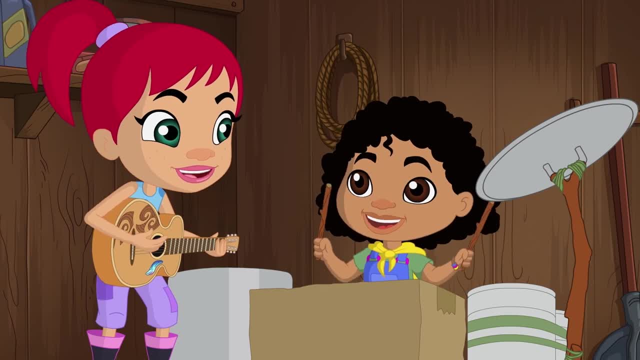 Jamming From a little tune down once been humming Humming, Now in the basement Mutes like strumming. Trumming Any melody, Any life, strumming Everything makes a different sound. You can make music from stuff that lies around. 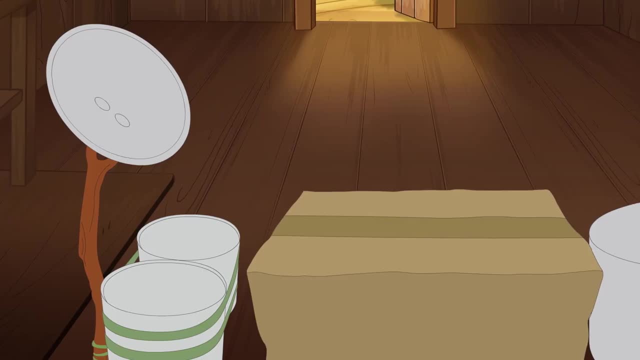 One, two, three, four. Testing testing: One, two, three. One, two, three. Can you hear us sing? A B C, A B C. Do you hear the sound when I sing, When I sing? 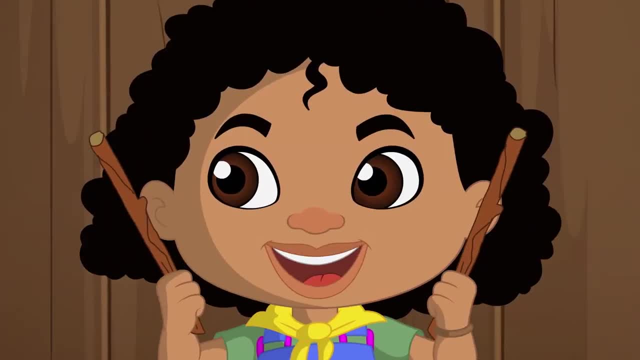 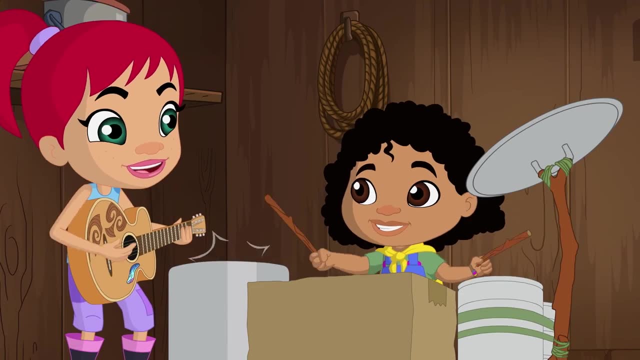 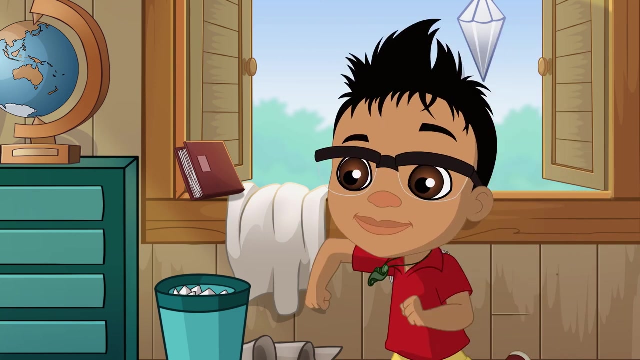 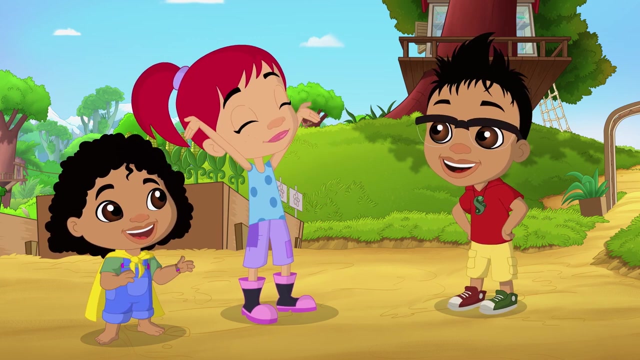 Through the air and down the string. One, two, three. Do you hear the sound when I sing, When I sing Yeah and down the string? Wow, that sounded wonderful Over. Yes, Henny, That was so much fun. 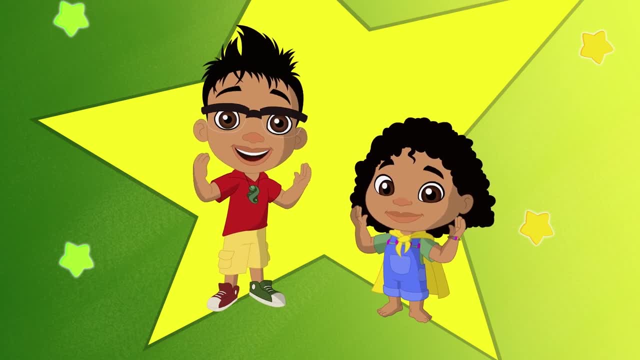 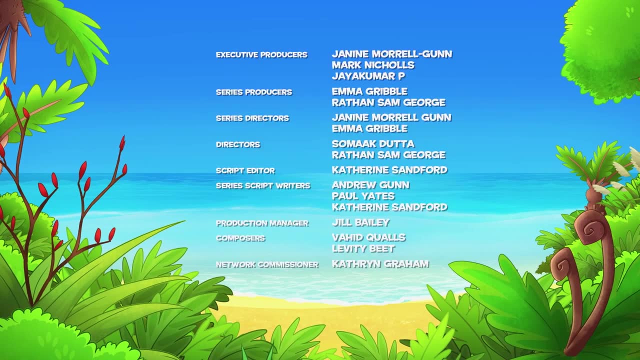 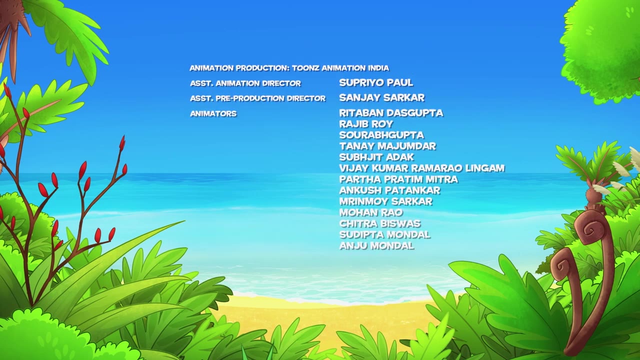 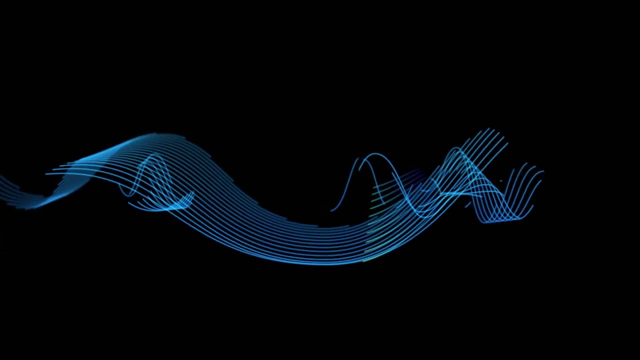 Yes, and you two sounded great. Mi hao, Awesome. Head to darwinandyouthcom for more. We'll see you next time.